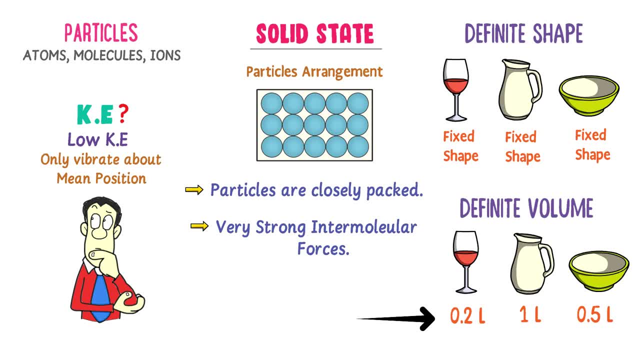 the glass is fixed 0.2 liter, volume of the jug is fixed 1 liter and volume of the pot is fixed 0.5 liter. Here let me ask you: can solids fill the container or any object? 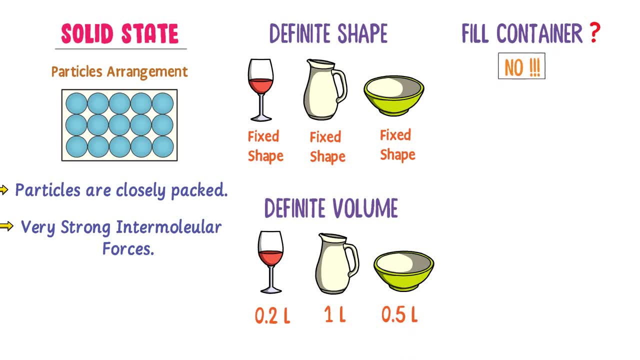 in which they are placed. The answer is no. Solids do not fill the container completely. For example, consider sugar or salt in this pot. It only occupies the required volume. It doesn't completely fill the object. Secondly, can we compress solids? The answer is again no. We cannot compress solids If 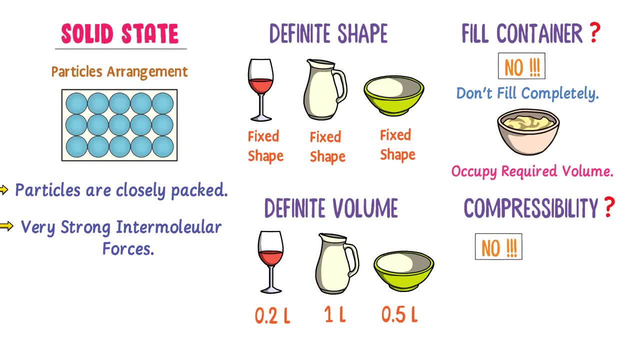 you think why? let me explain it. For example, consider this solid pot. The particles of this pot are closely packed together. There is no inter-spaces between them. Even if we exert force on it, we cannot compress it further. So we say that we cannot compress solids. 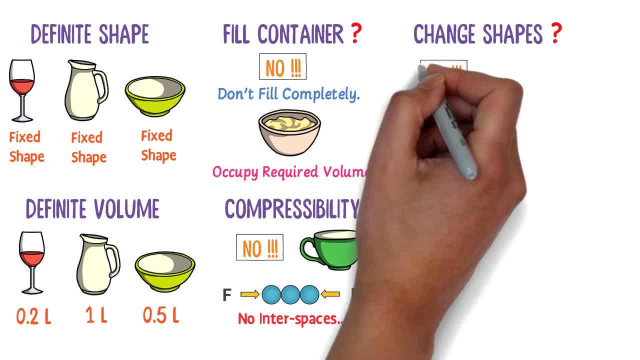 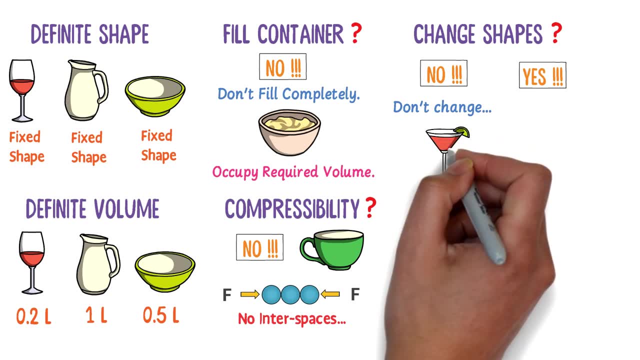 Thirdly, can solids change their shapes? The answer is no. We cannot compress solids. We cannot compress solids. We cannot compress solids. The answer is no and yes. Solids do not change their shapes by their own. For example, if you keep this glass here, it will not change its shape with the passage of time. 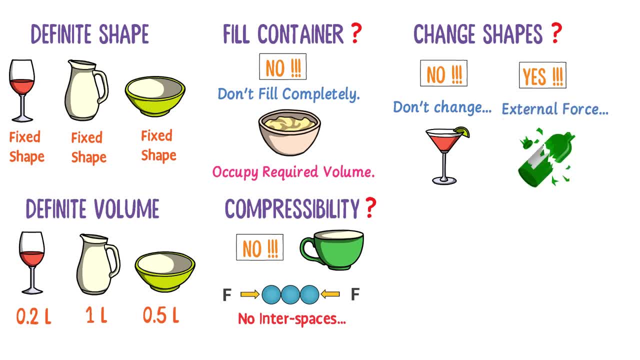 But if you exert external force on it, then solids change their shapes. They are broken into pieces. So solids do not change their shapes by their own, But they can change shapes under external forces. Also, remember that there are two main types of solids: Crystals. 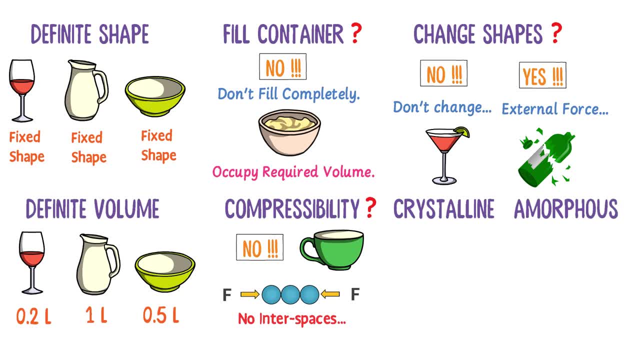 and Amorphous solids. In crystalline solids, particles are packed together in three-dimensional pattern or in regular pattern. For example, sugar, diamond, rock are crystalline solids, While in amorphous solids particles are not packed together in three-dimensional pattern. 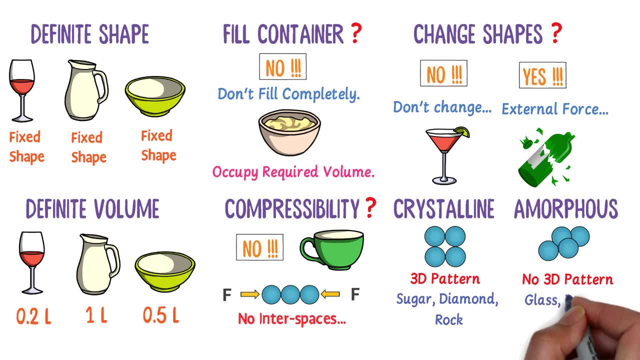 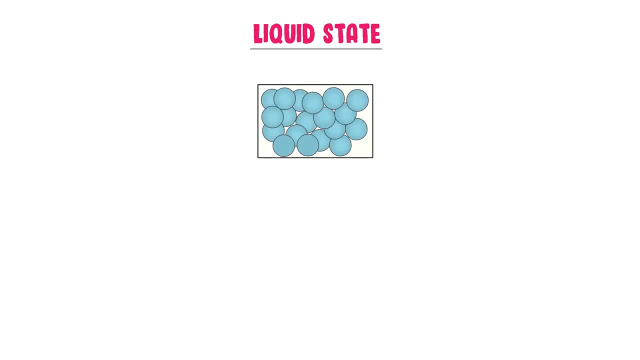 or in irregular pattern. For example, glass, plastic and gel are amorphous solids. So note it down, all these important points about solid state of metal. Now let me teach you about the liquid state of a metal. At microscopic level, this is: 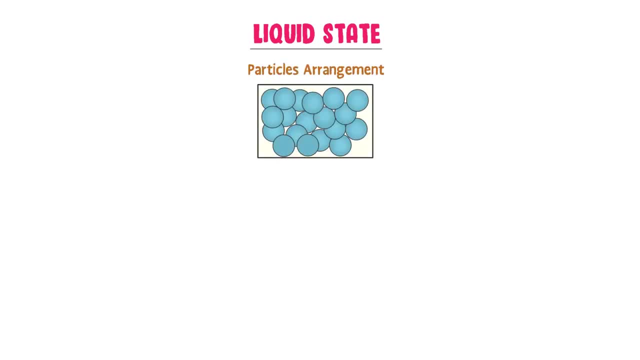 the arrangement of particles in liquid state. In liquid state particles are closely packed together, with no regular arrangement. The intermolecular forces between particles are strong but weak than those in solids. What about the motion or kinetic energy of particles in liquid state? 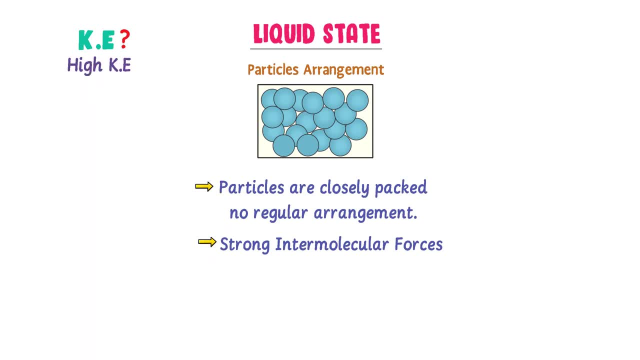 Well, the particles of liquid have high kinetic energy. I mean the particles of liquid slide over each other. In chemistry we say that particles of the liquids are in random motion or irregular motion. For example, consider water and this glass. The particles of water. 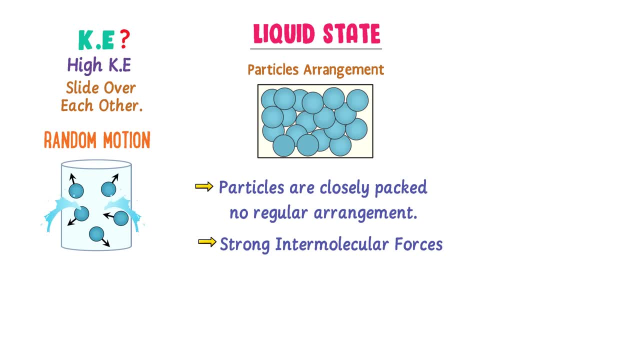 move in all directions and constantly collide with the walls of a glass. So we say that particles of the liquid have random motion or irregular motion. regular motion. On the other hand, liquids have indefinite shape. For example, consider one liter water in this object and one liter water in this object. In this object, the 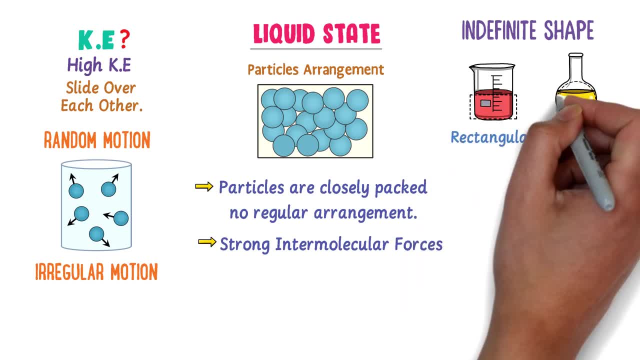 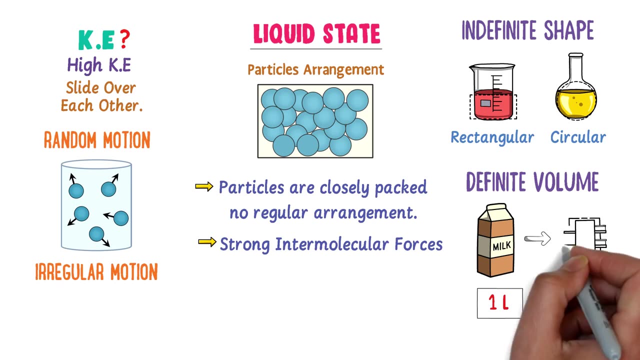 shape of water is rectangular, while in this object the shape of water is circular or spherical. So water changes its shape in different objects, While liquids have definite volume. For example, you buy one liter milk in the market and you bring it to the home. 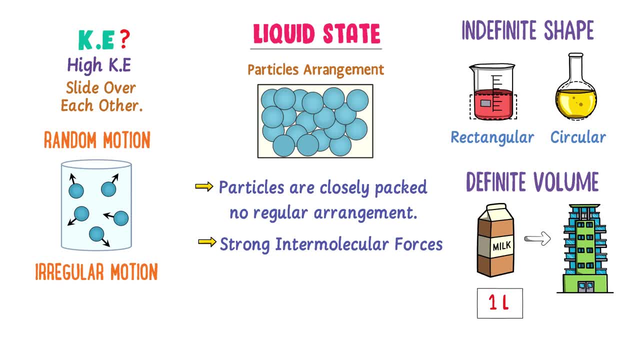 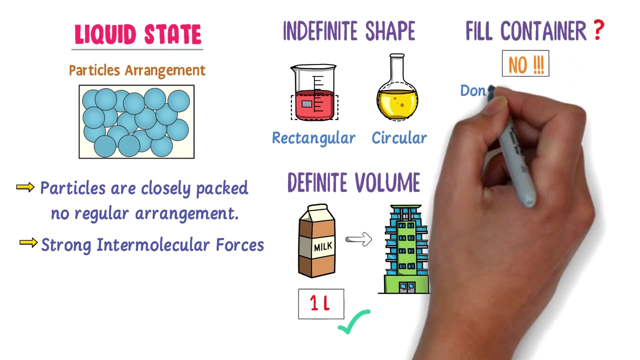 Does the volume or amount of milk change? The answer is no. The milk is still one liter in your home. So we say that liquids have definite volume. Here let me ask you: can liquids fill the container? The answer is no. Liquids do not fill the container completely. 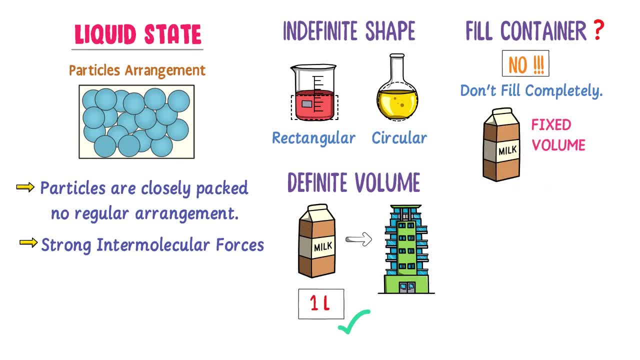 Because they have fixed volume. they occupy only the volume. Secondly, can we compress liquids? The answer is no. We cannot compress liquids because there is no interspaces between particles of liquid, due to which they are not compressed. Thus noted down all these important points about liquid. 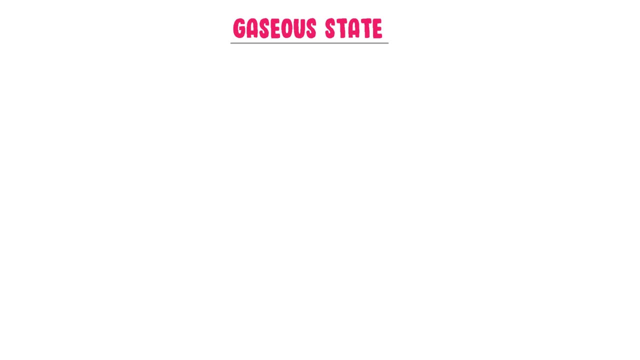 Now let me teach you about the gaseous state of a matter. At microscopic level, this is the arrangement of particles and gases In gaseous state. particles are separated with no regular pattern. The intermolecular forces between particles are very weak and gaseous.